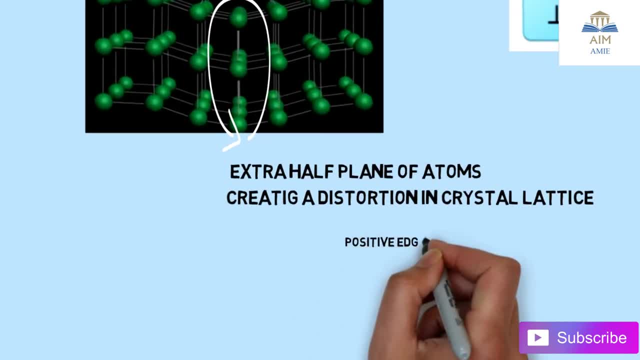 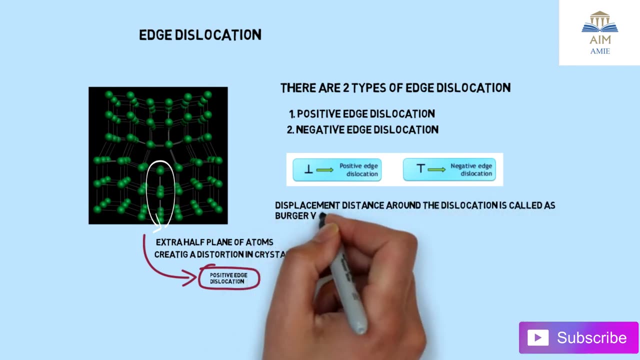 negative. so in this case the extra half plane atoms from the downward. so that's why this is the positive h dislocations. so you can see over here in this image this is the positive h dislocation. so the displacement distance around the dislocation is known as the berger vector. 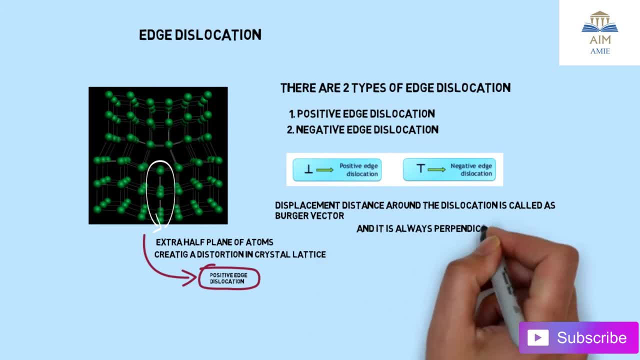 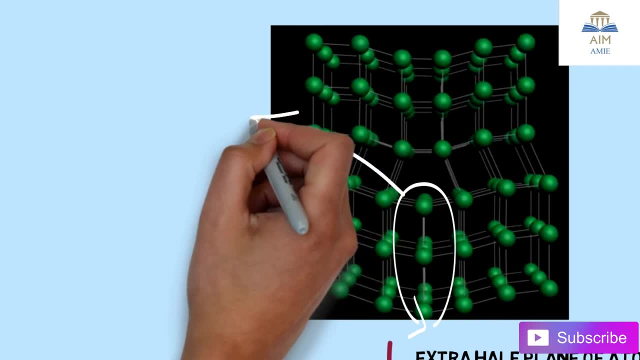 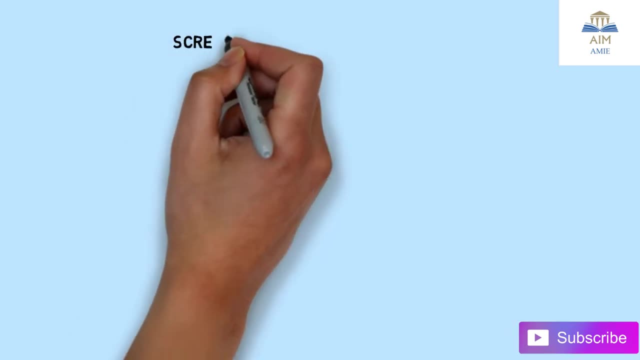 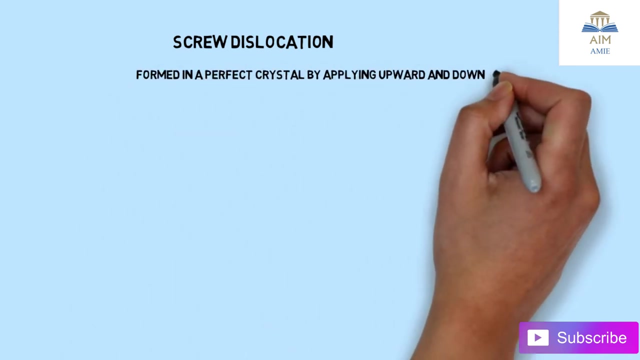 and it is always perpendicular to the displacement, sorry, the dislocation line. so in this image, this is the line that is the displacement, this is the dislocation line, that is displacement distance. so next one is the screw dislocation. so the screw dislocation is formed in a perfect crystal by applying upward and downward shear. 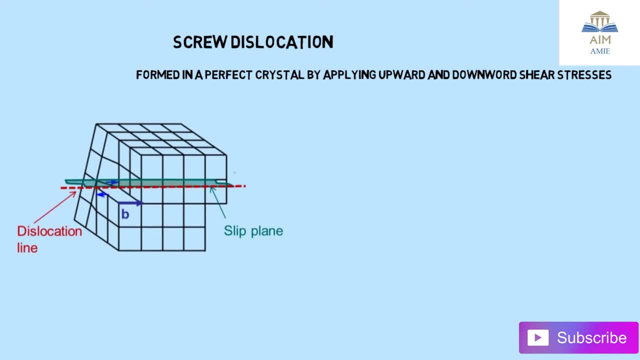 stresses. so shear stresses are the shear stresses of the dislocation. so the shear stresses of the dislocation is very important term. in this image you can see that there is a slip plane. dislocation line is there. there is b. the b is the berger vector. okay, so guys, what is the berger vector? 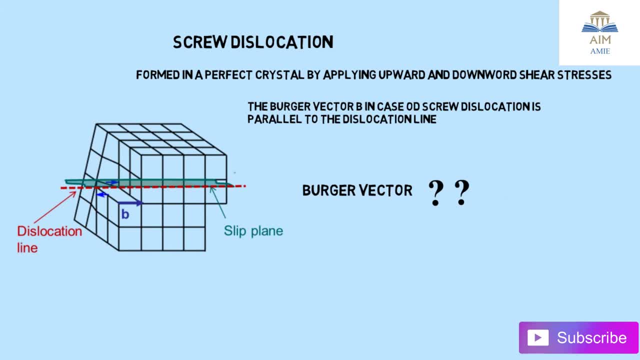 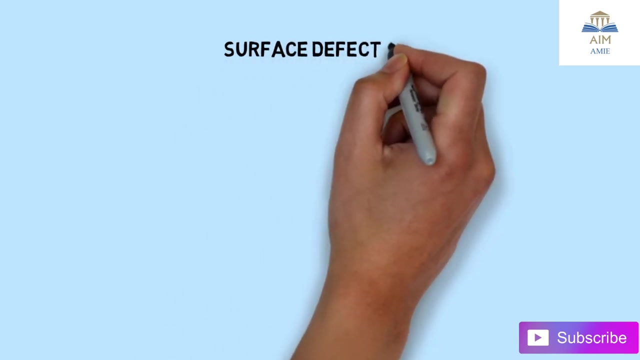 so berger vector is the characterizes the dislocation line. basically it indicates whether the dislocation line is h or screw dislocation. a berger circuit is the atom or atomic path which forms a closed circuit, which is known as a berger circuit. next one is the surfact defect. so this mainly comprises with the boundaries. 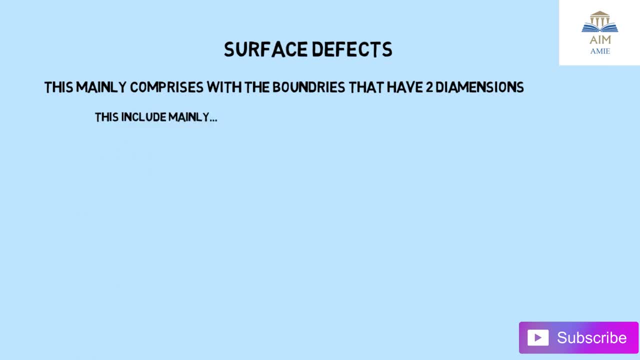 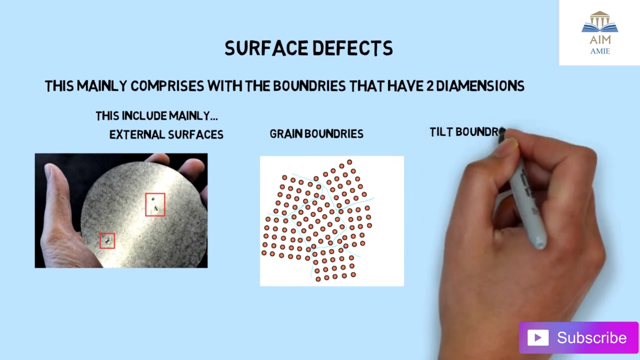 that have two dimensions. this includes mainly, basically, the external surfaces. so in this image you can see that over there on the surface of the plate, there are some defects. second one is the grain boundaries. I mean, in the perfect crystals the grain boundary should be linear, or in this image you can see that this is a distorted grain boundaries. the next one is the 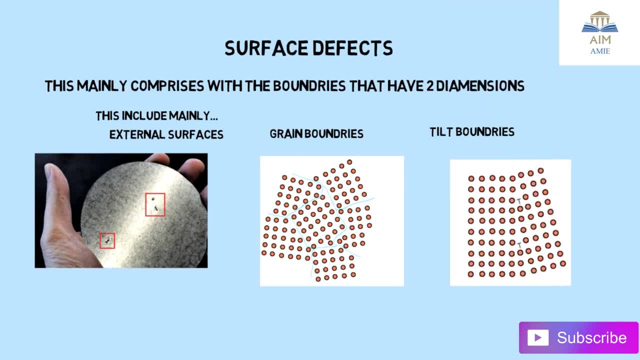 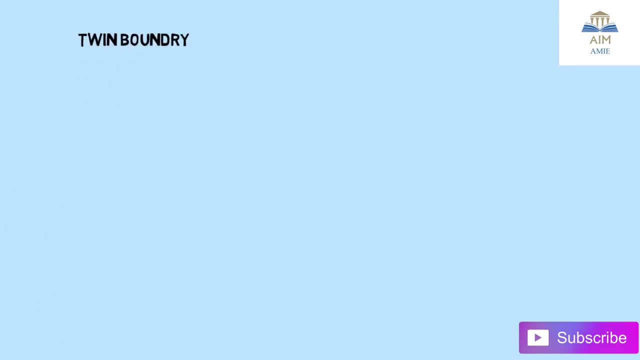 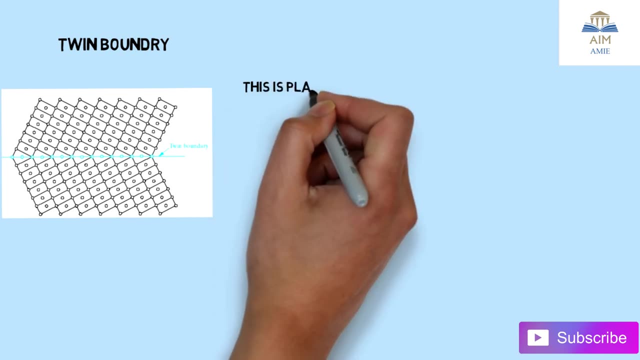 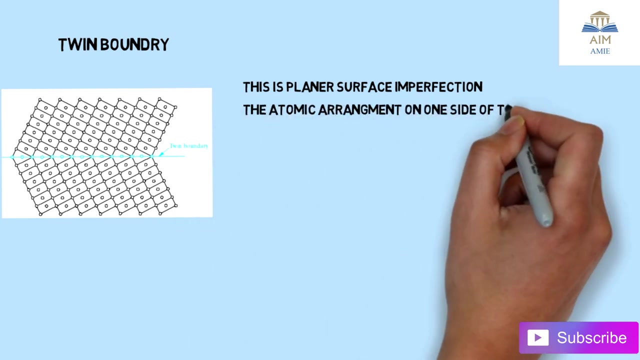 tilt boundaries. so these are the angular displacement. so next one is in the surfact defect, that is twin boundary basically. so twin boundary is nothing but the mirror like structure. you can see that. so this is the planar surfact imperfections. planar is very important word over here, the atomic arrangement of one side.